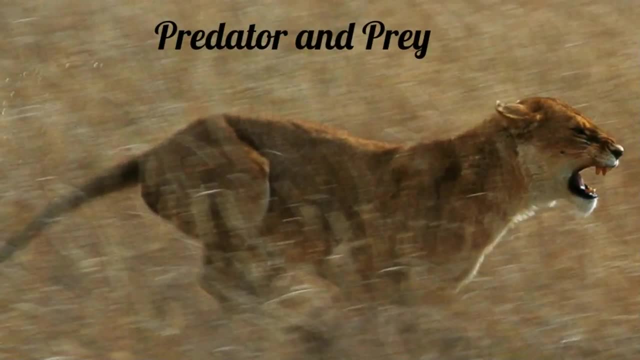 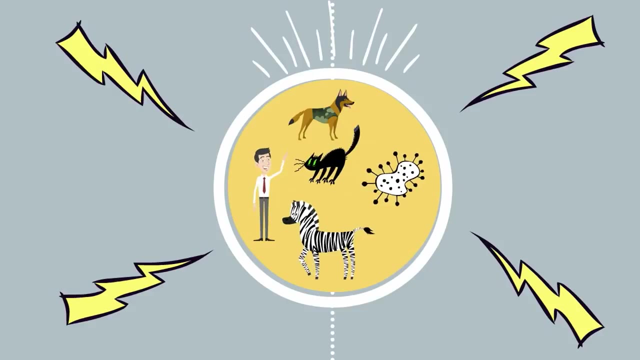 Welcome to MooMooMath and Science. In this video, I would like to talk about the interaction of predator and prey. All living things require energy. However, living things get their energy in different methods. Sometimes one individual consumes another individual, A term used to 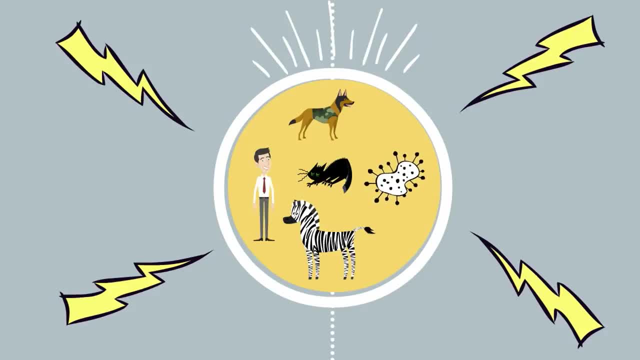 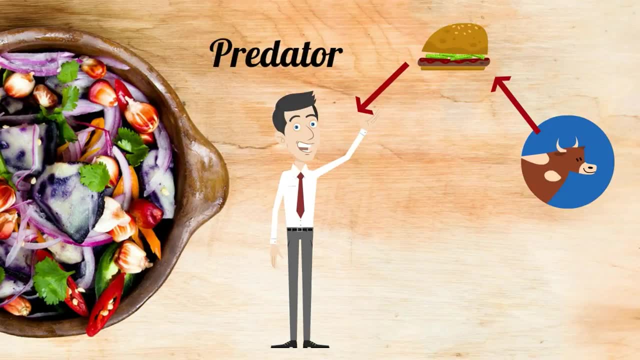 describe this interaction is called predator and prey. The individual that is consuming the other is the predator and the living thing that is consumed is the prey. Living things can be classified into two large categories: Autotrophs and Heterotrophs. Autotrophs generate 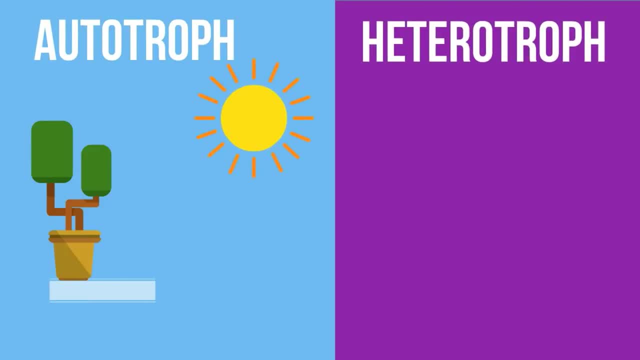 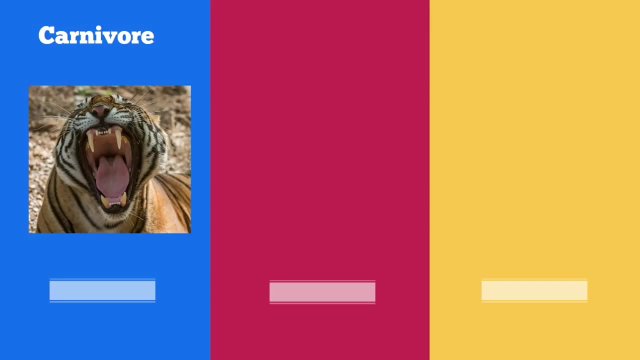 energy from the sun through a process called photosynthesis. Examples include plants and phytoplankton. Heterotrophs must consume living things for energy. Heterotrophs can be further divided into carnivores, which consume other animals- herbivores. 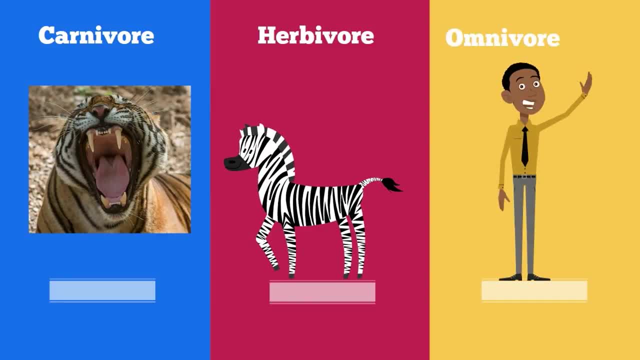 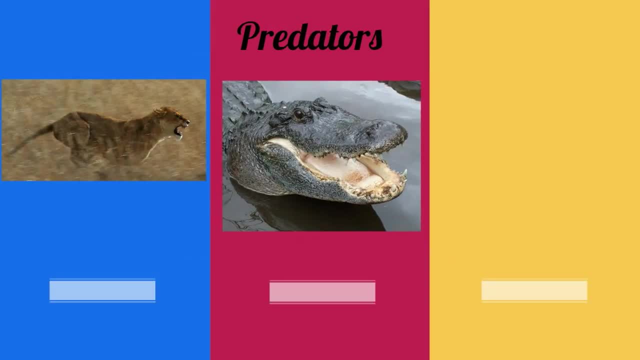 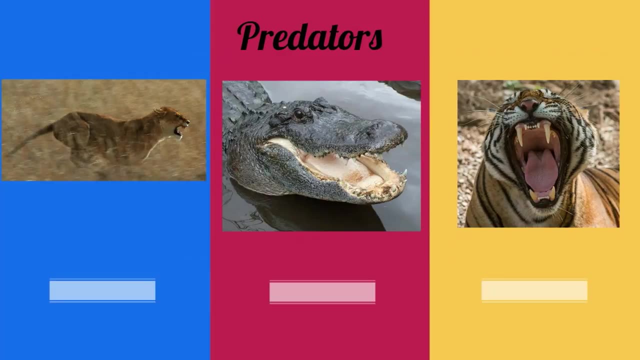 which consume plants, and omnivores, which consume both plants and animals. Many people think of lions, alligators or tigers as predators, But there is a huge number and variety of different predators in a predator and prey interaction. Take a look at this amoeba. This: 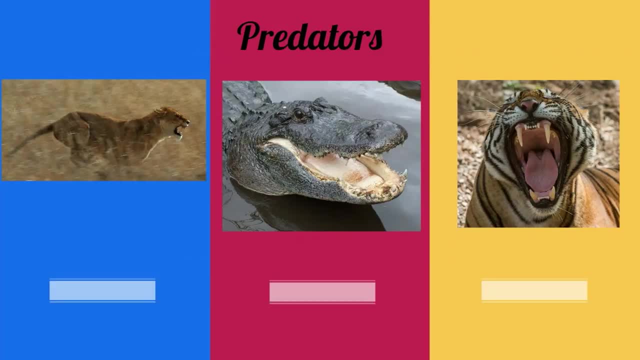 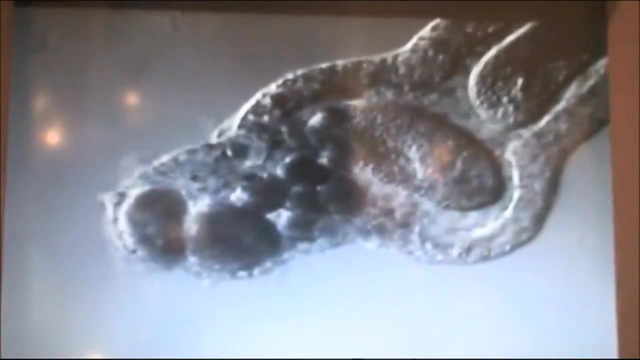 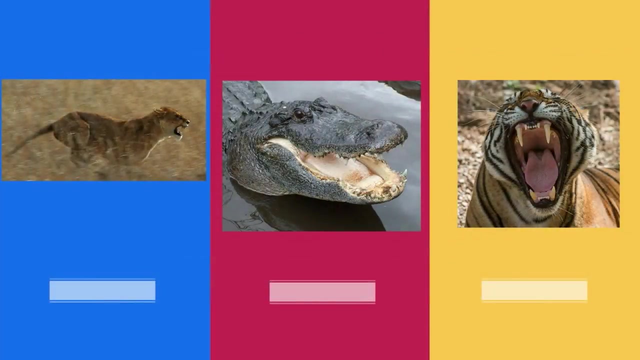 predator, it can consume a lot of food. What if this predator only eats this bush like a guava, which is the predator, consuming a paramecium, which is the prey? Watch this praying mantis attack its prey Last. finally, this may seem strange, but even this cow eating the grass is a predator. 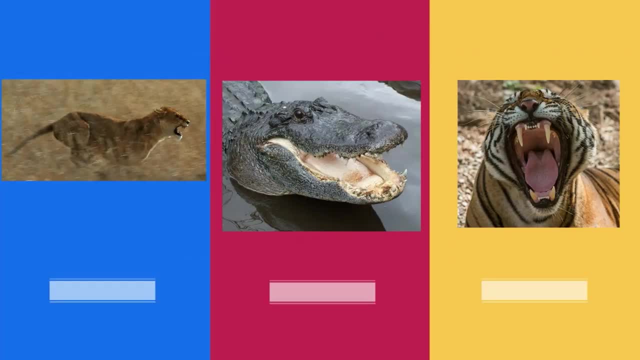 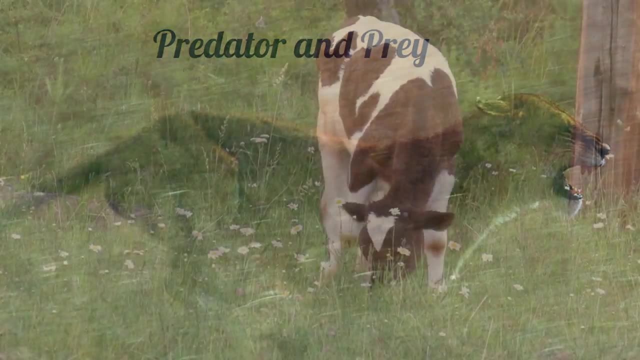 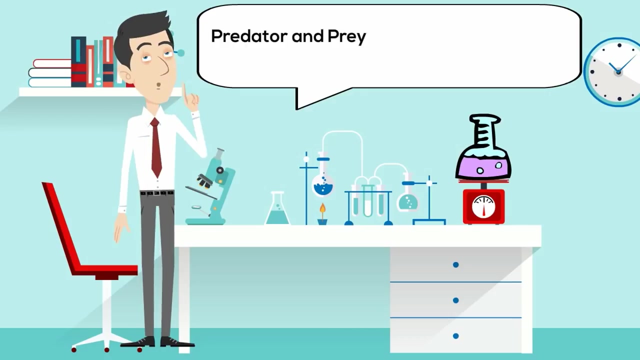 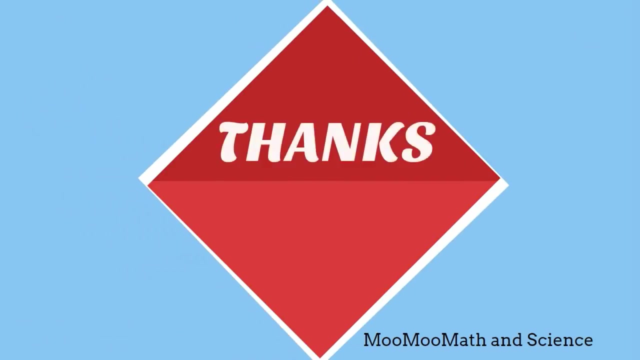 This Syringa Heaven, Heterophys, predator- prey interaction. The cow is the predator and the grass is the prey.